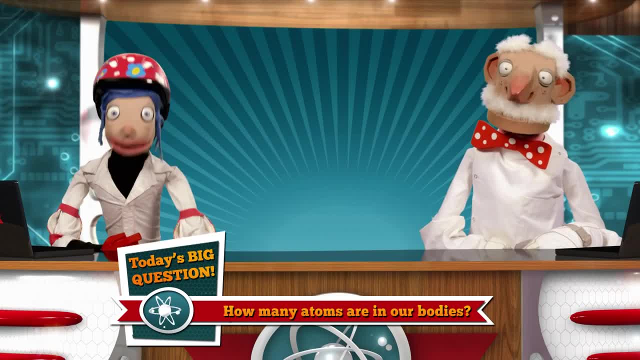 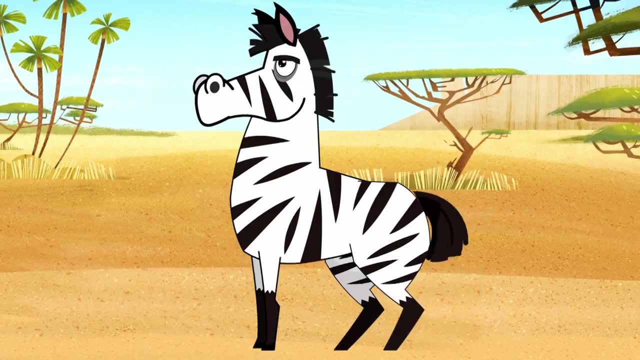 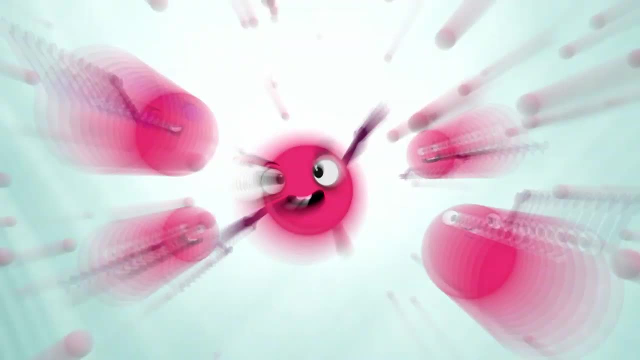 Today we're asking how many atoms are in our bodies. Atoms are the fundamental building blocks of our universe, and everything you see around you is made of atoms: Buildings, animals, water, air. Ooh, Careful. Atoms are unimaginably tiny and contain even smaller particles called protons, neutrons and electrons. 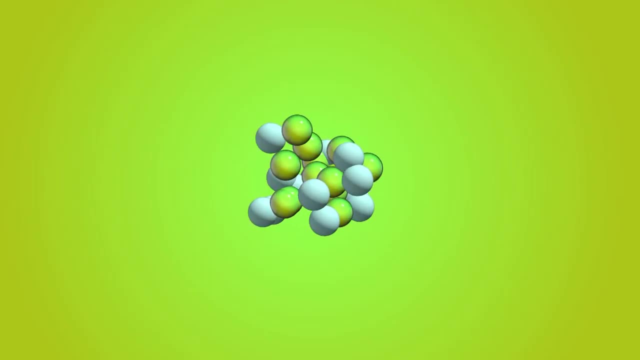 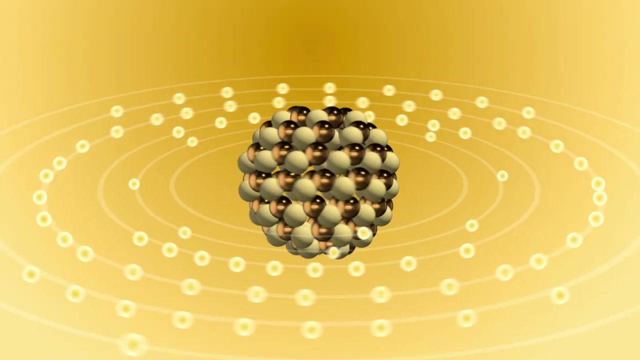 Depending on the number of protons in an atom, it takes on a different form known as a chemical element. So, for example, atoms with eight protons make oxygen, 20 make calcium and 79 make gold. Hang on a sec though. 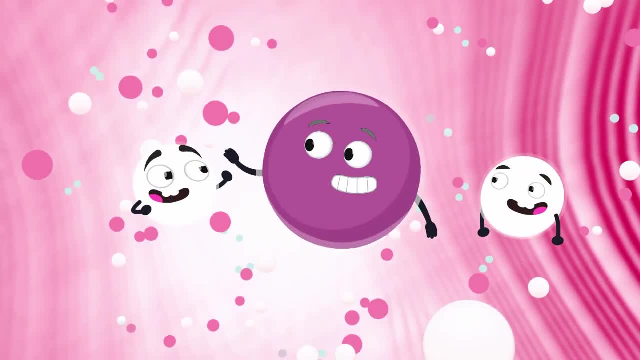 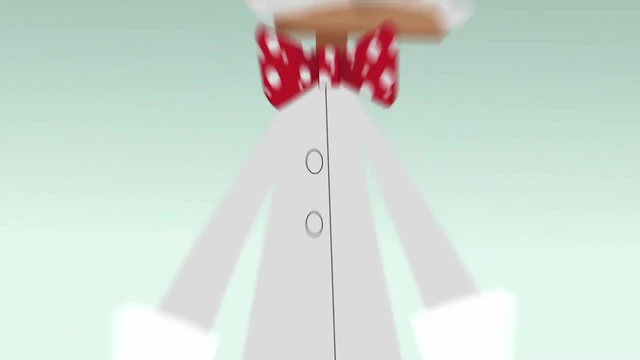 How are we made of those tiny little atoms In nature? atoms come together to form molecules, which form cells, then tissues, organs and eventually living organisms like us. Whoa, that's incredible, Dr Knowles. Whoa. 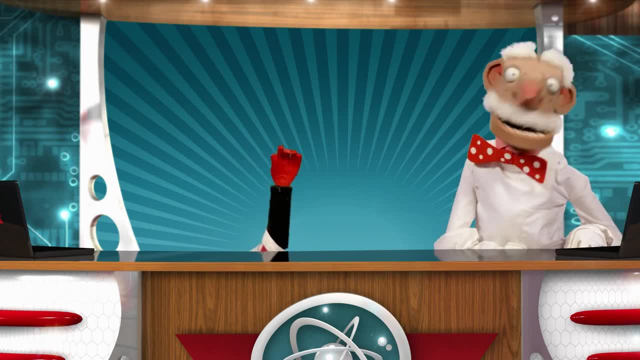 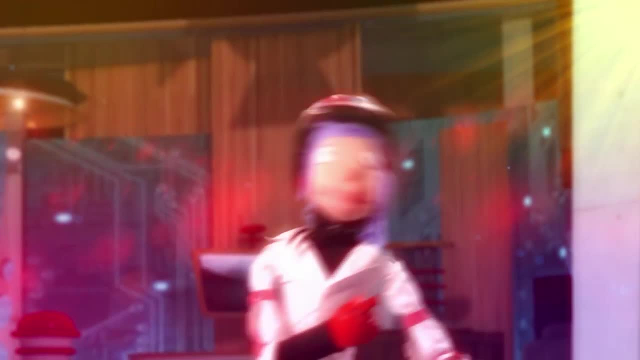 Dr Knowles Down here. Heh, I think it's time for a break. I'm clear. Oh no, This is the worst part. It's actually not that bad once you get moving. Come on, Dr Knowles, you're missing out. they're fine. 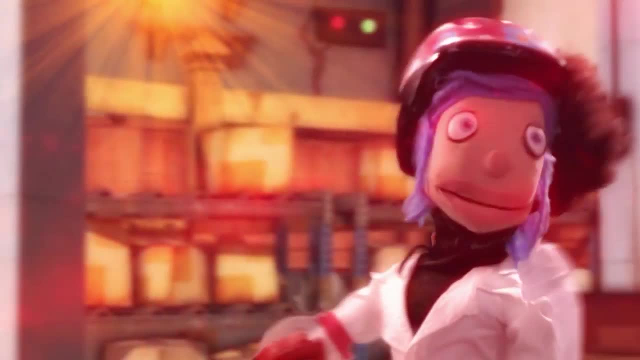 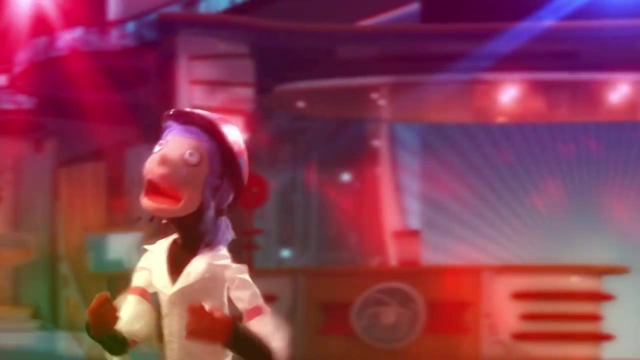 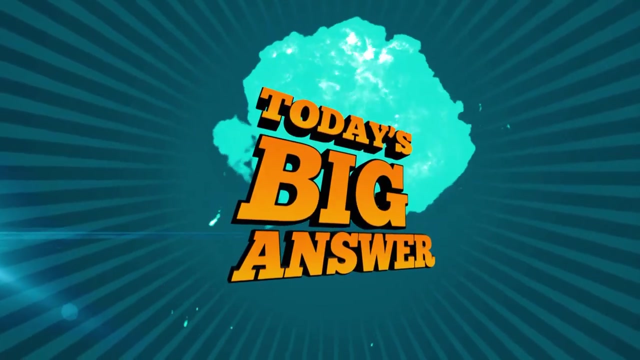 Hooray, Spin around. I think I'm getting the hang of this. Yeah, yeah, I think I'm doing it. I'm finally skating. Whee Positions everyone. Ah, Abracadabra, Today's Big Answer. 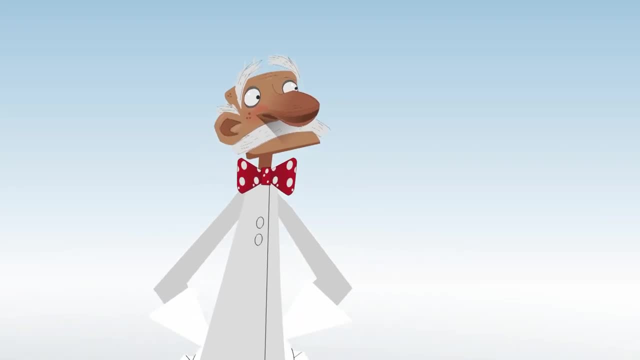 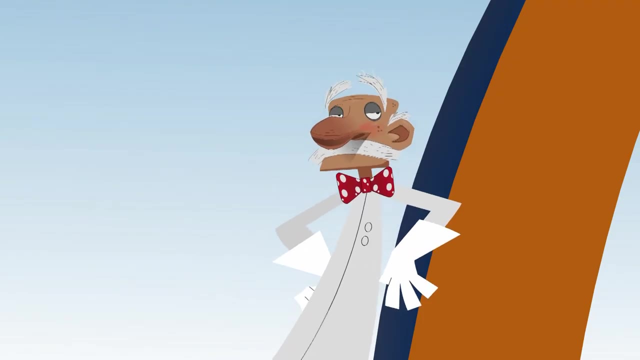 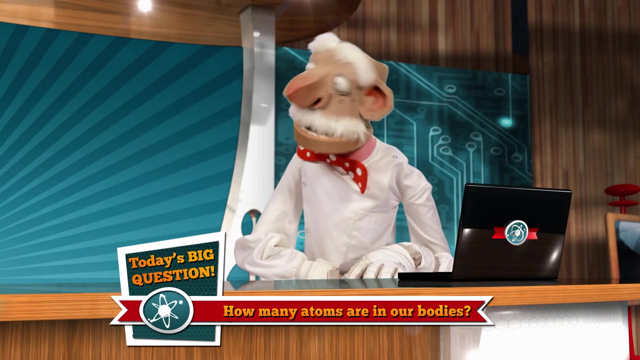 So tell us, Dr Knowles, how many of these teeny, weeny little atoms are there in our bodies? The body of an average adult human being will contain about seven billion billion billion atoms. That's a seven followed by twenty seven zeros. 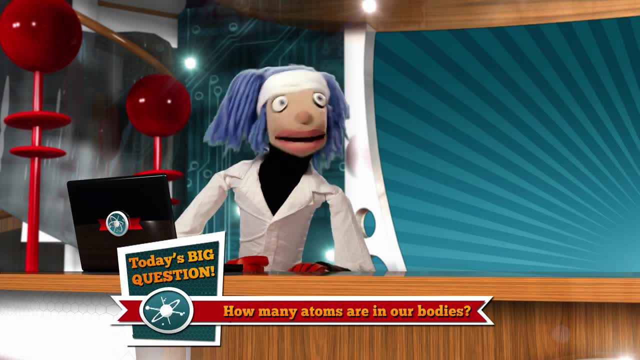 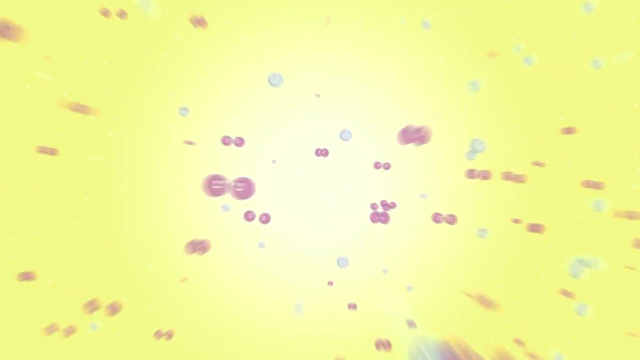 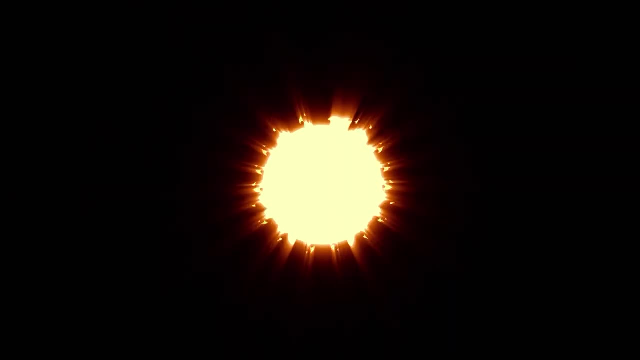 Now, that's a big, big, big number. Tell us, Doctor, where do they all come from? Deep in the cores of stars, atoms are fused together with lighter elements, fusing to form heavier ones. Hydrogen is fused into helium, helium into carbon and so on. When a star 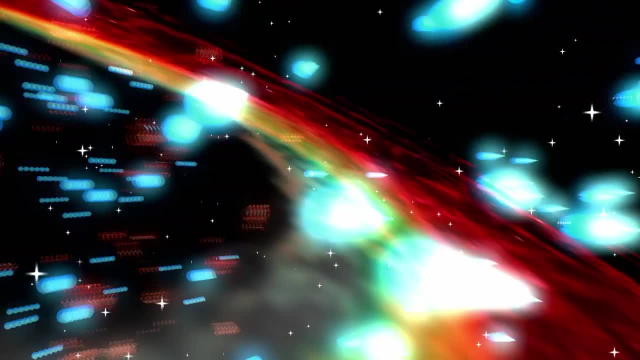 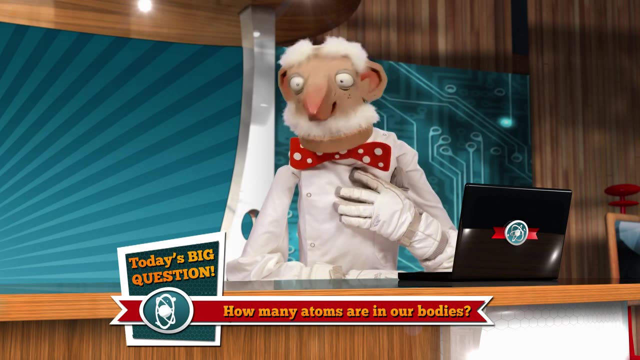 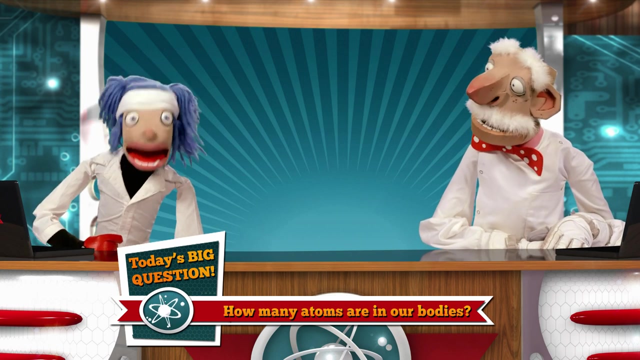 dies, it fires these newly formed elements out into the universe where they combine to make up all of the matter in the world around us. So we're actually made from stars. Pretty amazing, right? I think that's the coolest thing I've ever heard, Dr Knowles.